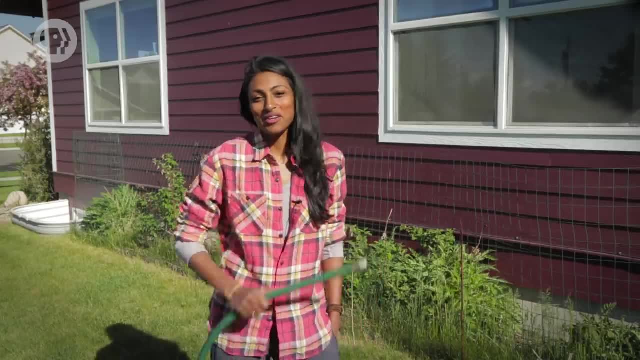 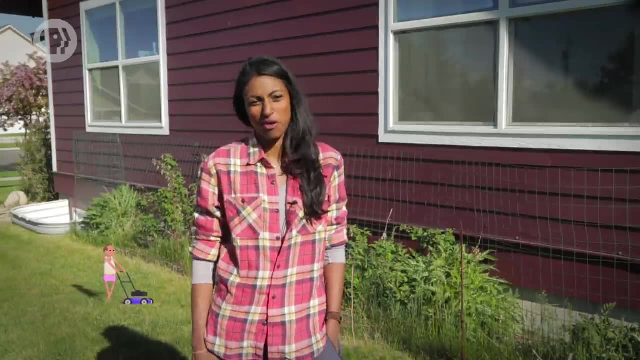 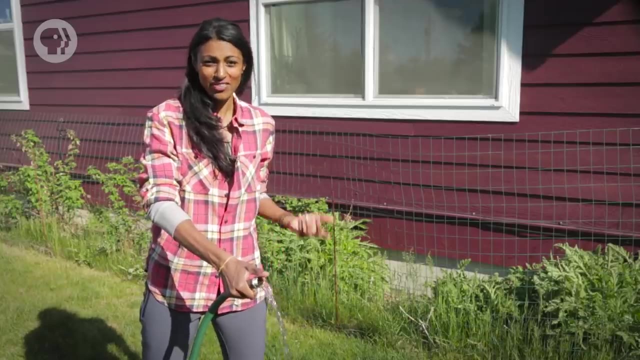 You know what can be kind of peculiar and surprising? The fact that whenever you want to shoot outside, everyone decides to mow their lawn. You know what else can be kind of peculiar and surprising? Water, And in the right circumstances, I could even take 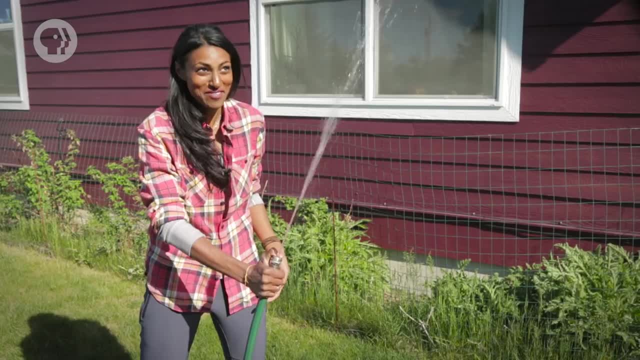 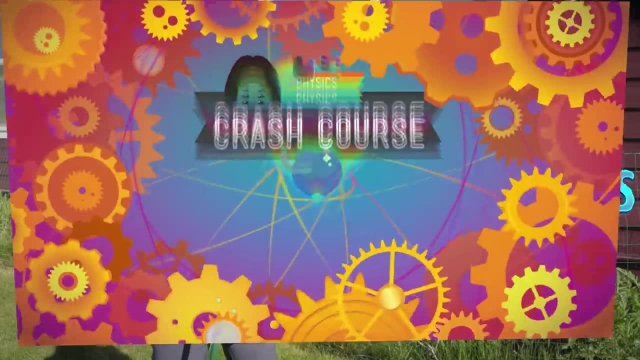 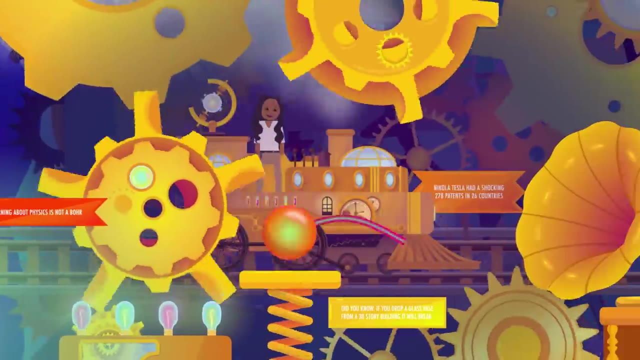 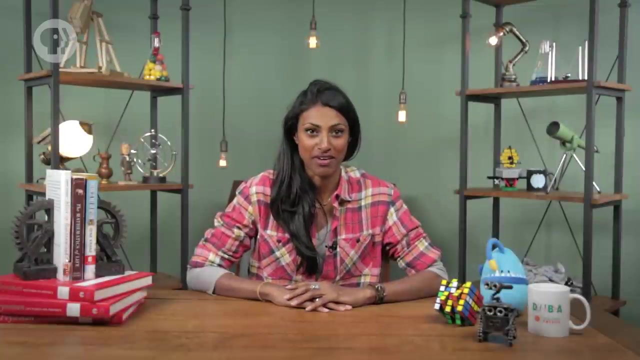 water that's flowing down and spurt it straight up. How All of these things are possible? thanks to the study of the flow of fluids, known as fluid dynamics. By now, you've picked up on the fact that, even though we live in the physical universe, 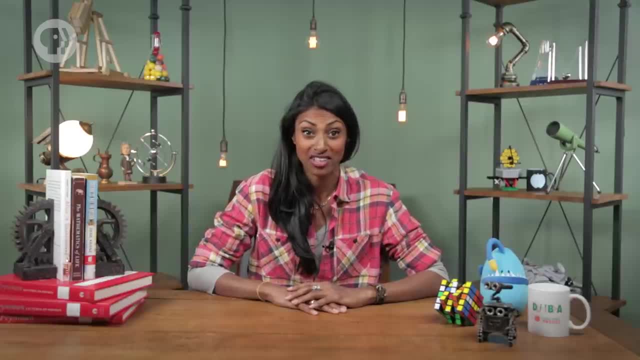 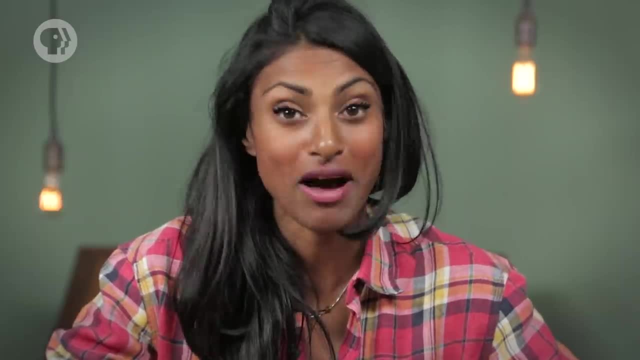 describing the rules of the universe sometimes requires us to pretend that certain things aren't happening. By the time we rolled a bunch of stuff down a ramp and pretended that there was no kinetic friction. the same is true when we talk about fluids, Because fluids in motion are… dynamic. 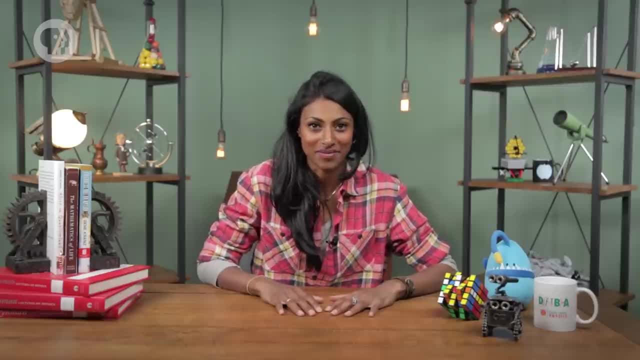 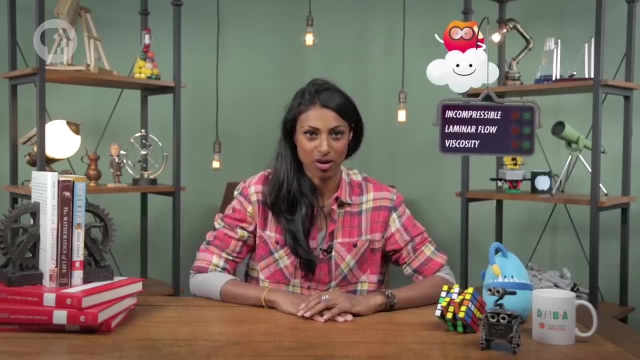 And there are many, many things going on in and around them all at once. So, in order to grasp the essentials of fluid dynamics, let's just do some pretending, shall we? For one thing, we're going to consider the fluids in our examples to be incompressible. 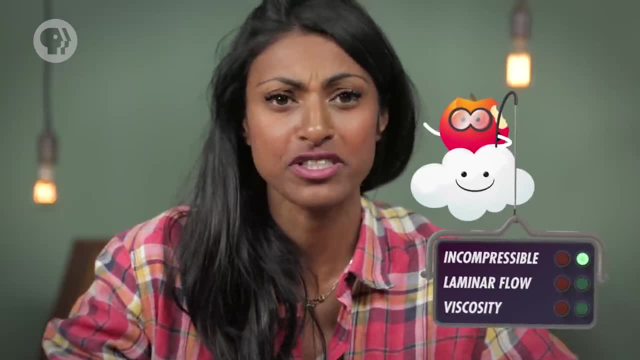 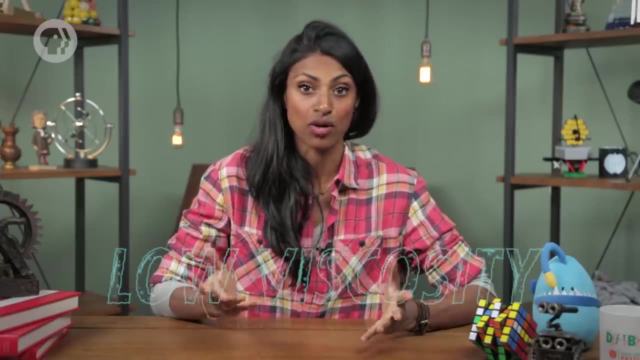 meaning that their densities won't change. We're also going to assume that fluids flow perfectly smoothly and have no viscosity. You've probably heard of viscosity before. When a fluid flows easily like water, we say that it has low viscosity. Fluids that don't flow as easily like honey have. 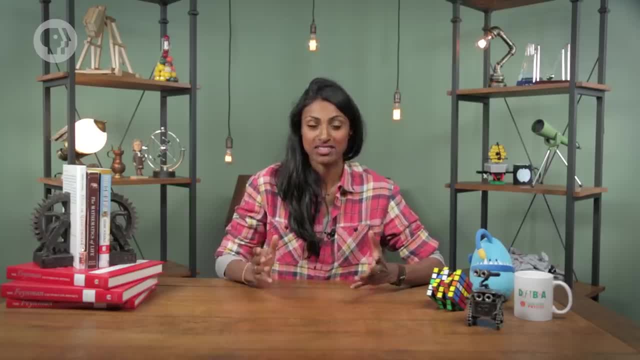 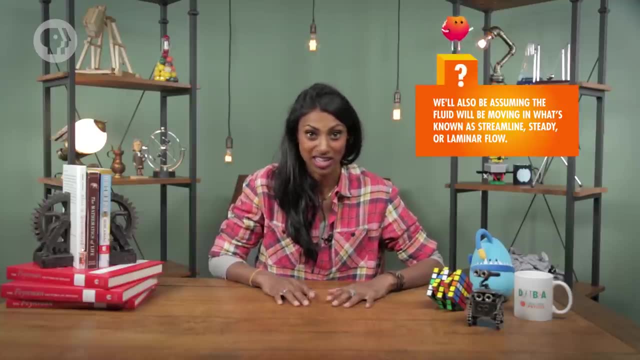 a higher viscosity And, much like kinetic friction does in moving objects, viscosity tends to complicate things in moving fluids, which is why we're going to generally pretend that the fluids we're studying don't have any. Now say you have some water which exists under all of these hypothetical conditions. 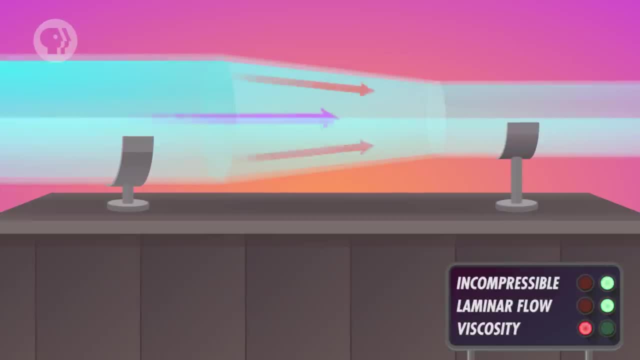 in a pipe moving along smoothly. This pipe narrows about halfway through so that one end is more narrow than the other. This shape is going to affect some of the properties of the water's flow as it flows. This shape is going to affect some of the properties of the water's flow as it flows. 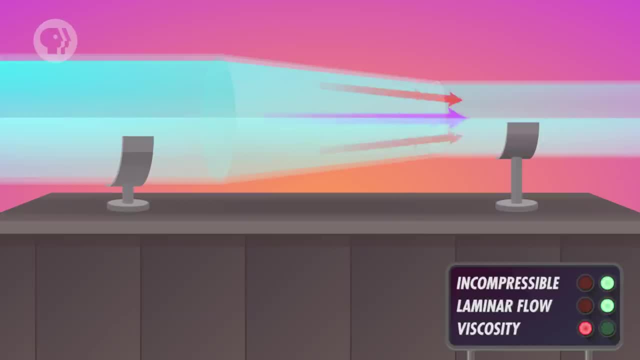 This shape is going to affect some of the properties of the water's flow as it passes through the more narrow side of the pipe compared to the wider side, But one thing that won't change is the mass of water that's moving through any given 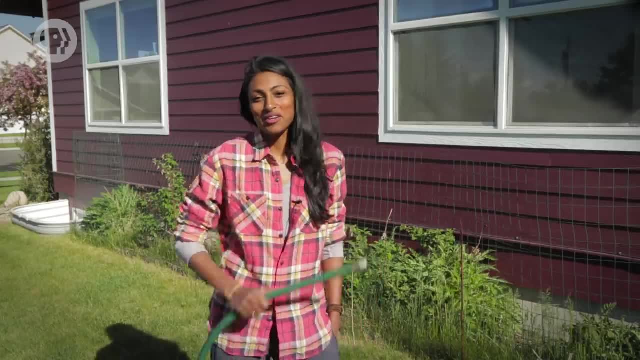 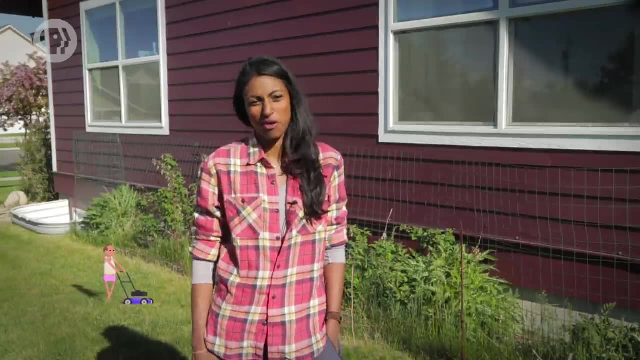 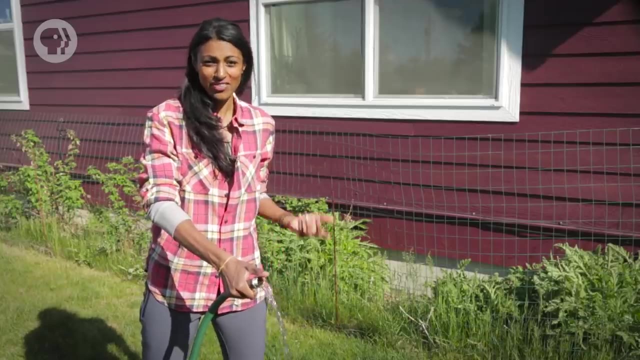 You know what can be kind of peculiar and surprising? The fact that whenever you want to shoot outside, everyone decides to mow their lawn. You know what else can be kind of peculiar and surprising? Water, And in the right circumstances, I could even take 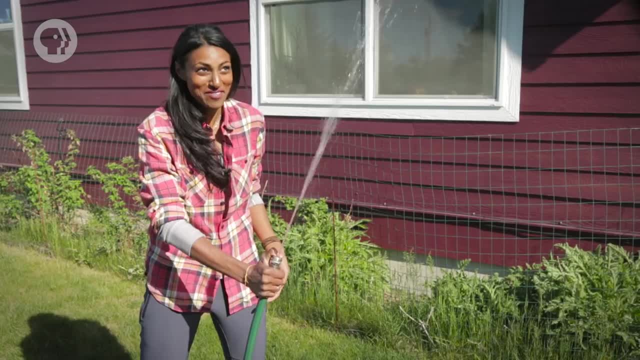 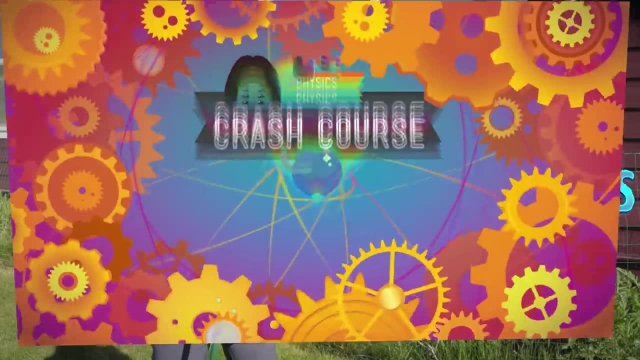 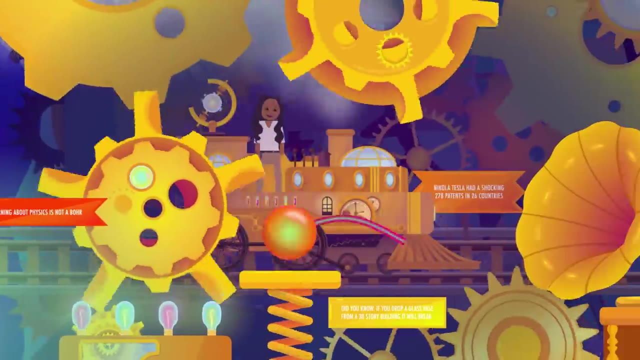 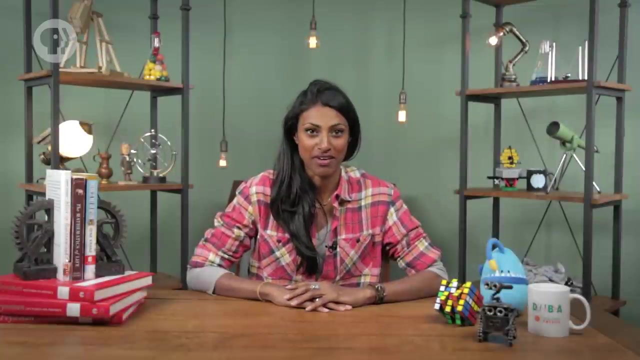 water that's flowing down and spurt it straight up. How All of these things are possible? thanks to the study of the flow of fluids, known as fluid dynamics. By now, you've picked up on the fact that, even though we live in the physical universe, 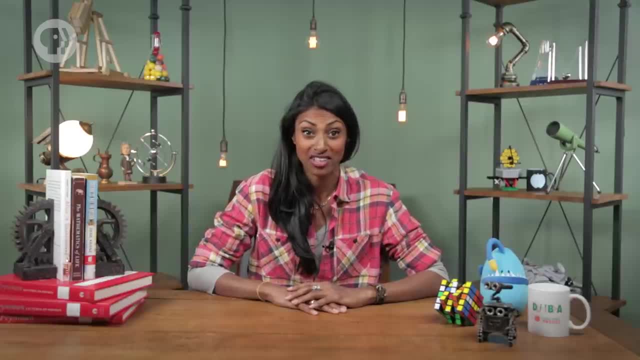 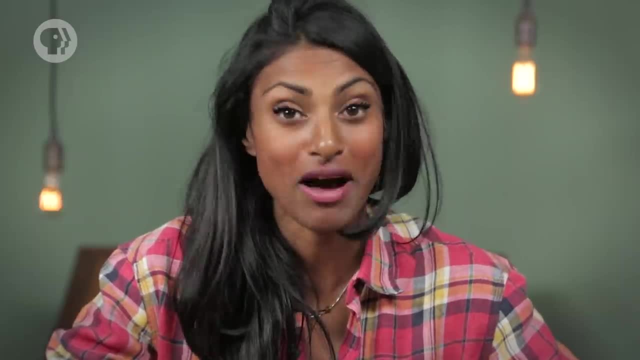 describing the rules of the universe sometimes requires us to pretend that certain things aren't happening. By the time we rolled a bunch of stuff down a ramp and pretended that there was no kinetic friction. the same is true when we talk about fluids, Because fluids in motion are… dynamic. 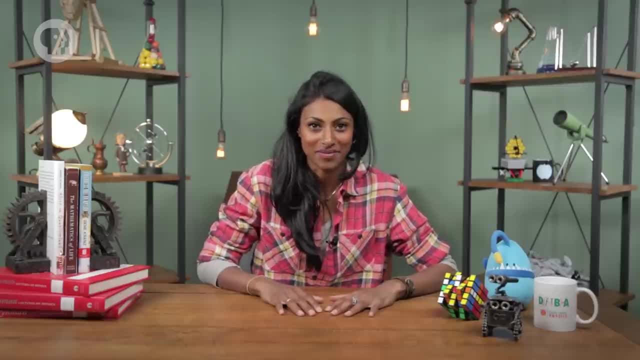 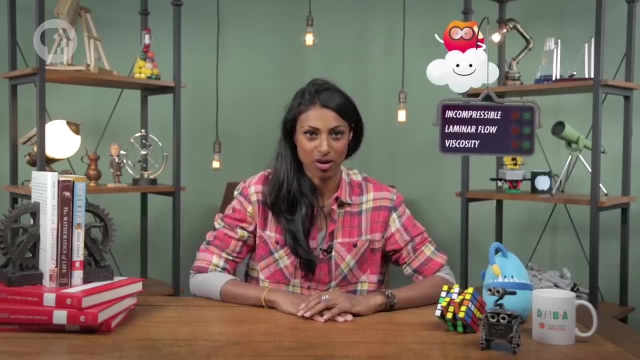 And there are many, many things going on in and around them all at once. So, in order to grasp the essentials of fluid dynamics, let's just do some pretending, shall we? For one thing, we're going to consider the fluids in our examples to be incompressible. 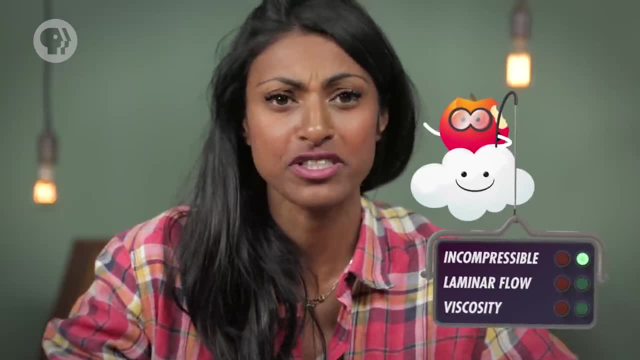 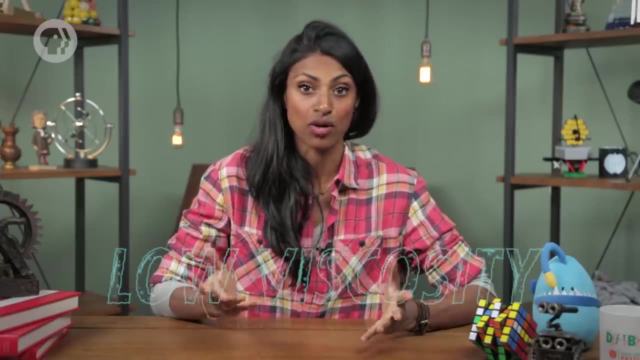 meaning that their densities won't change. We're also going to assume that fluids flow perfectly smoothly and have no viscosity. You've probably heard of viscosity before. When a fluid flows easily like water, we say that it has low viscosity. Fluids that don't flow as easily like honey have. 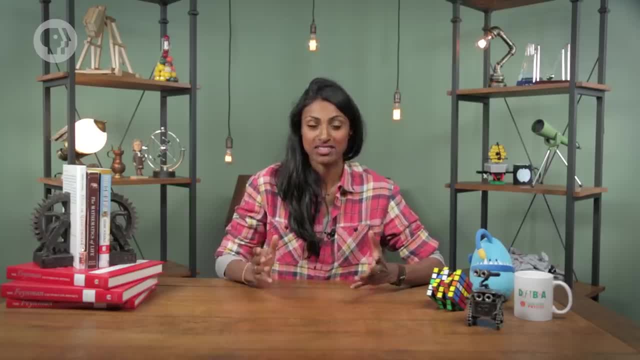 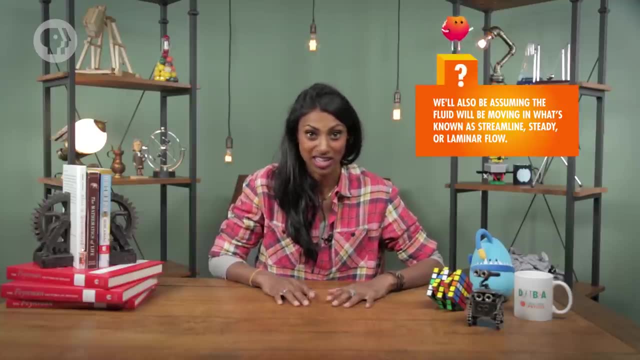 a higher viscosity And, much like kinetic friction does in moving objects, viscosity tends to complicate things in moving fluids, which is why we're going to generally pretend that the fluids we're studying don't have any. Now say you have some water which exists under all of these hypothetical conditions. 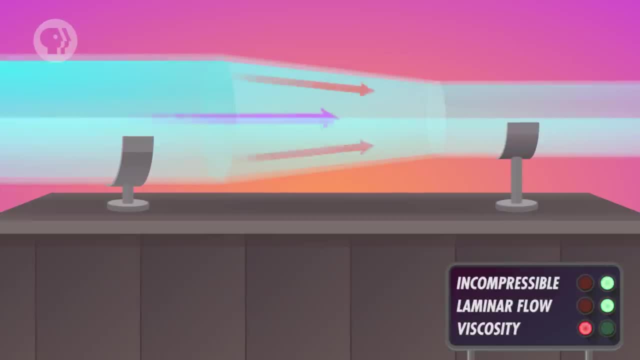 in a pipe moving along smoothly. This pipe narrows about halfway through so that one end is more narrow than the other. This shape is going to affect some of the properties of the water's flow as it flows. This shape is going to affect some of the properties of the water's flow as it flows. 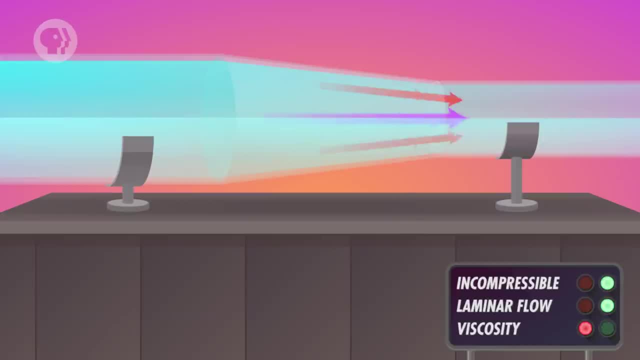 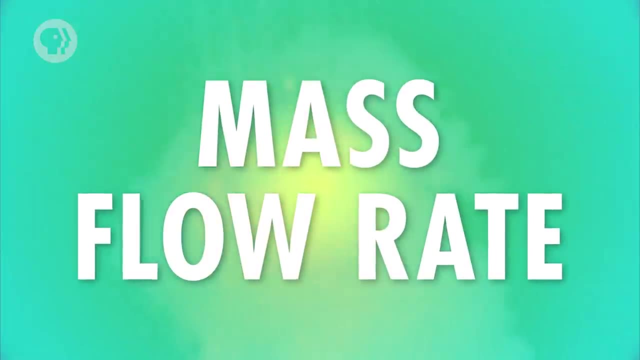 Thus the water passes through the more narrow side of the pipe compared to the wider side, But one thing that won't change is the mass of water that's moving through any given area of the pipe over time. This is called the mass flow rate, and it's always going to be the same everywhere in 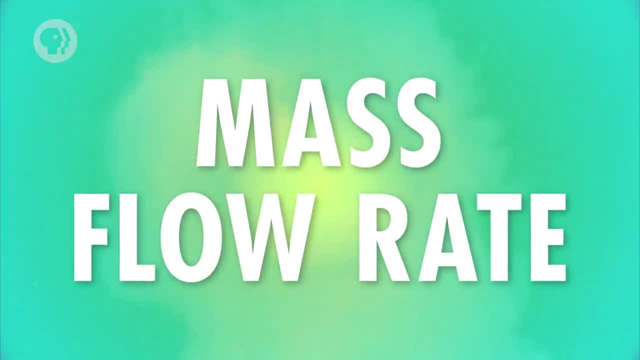 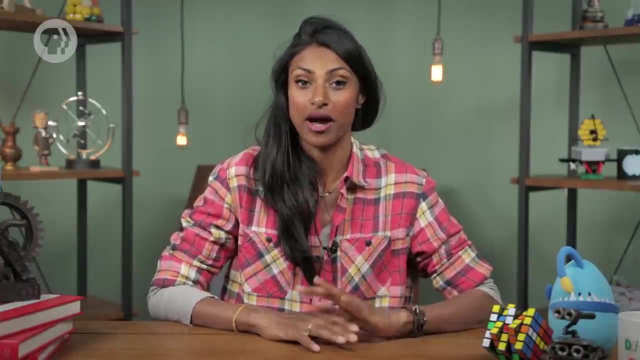 area of the pipe over time. This is called the mass flow rate, and it's always going to be the same everywhere in the pipe. That's just because, as the water flows through the pipe, it pushes along the water in the rest of the pipe too. 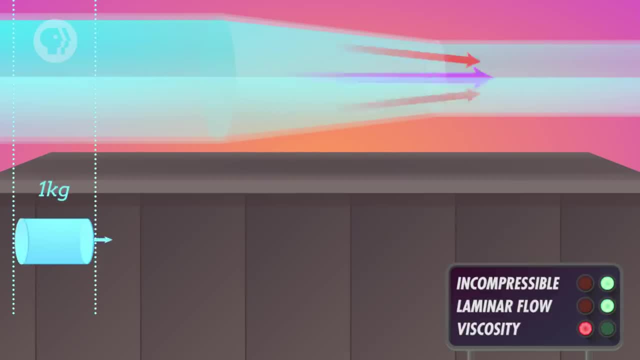 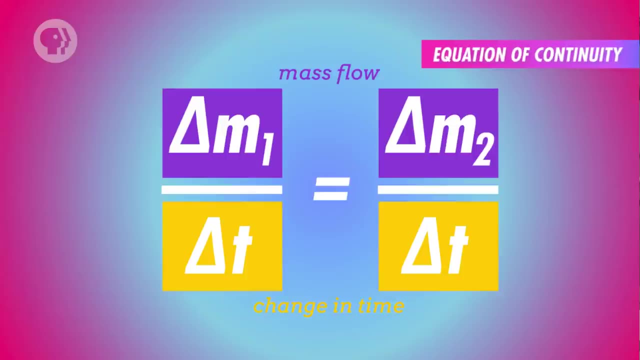 So if one part of the pipe has, say, a kilogram of water moving through it every second, the rest of the pipe also has to have a kilogram of water moving through it every second. This fact that the mass flow rate at one point of the pipe is lower than the other. 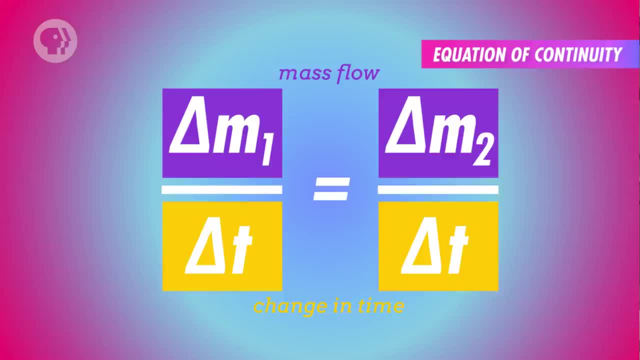 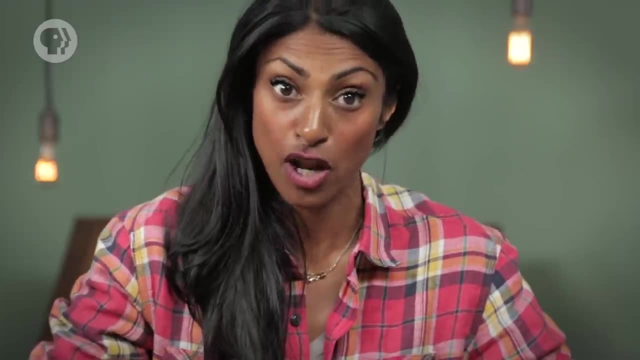 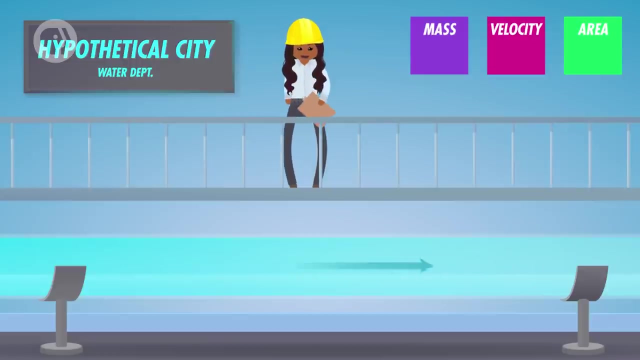 pipe will be equal to the mass flow rate at any other point is called the equation of continuity, And it can tell you a lot about the relationship between the velocity of a fluid and the cross-sectional area of the pipe that it's flowing through. Let's say you're an engineer for the water department of Hypothetical City and you need to understand the mass flow rate of hypothetical water that's going through a certain point in your underground pipe system. 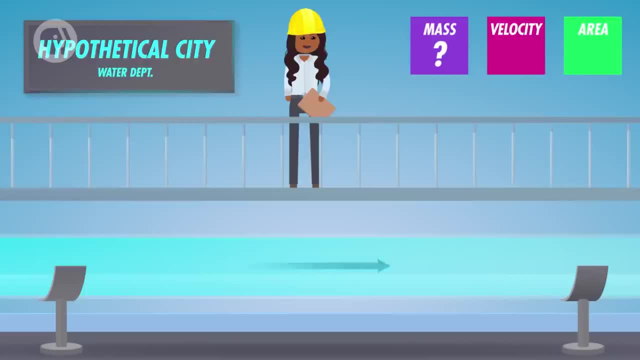 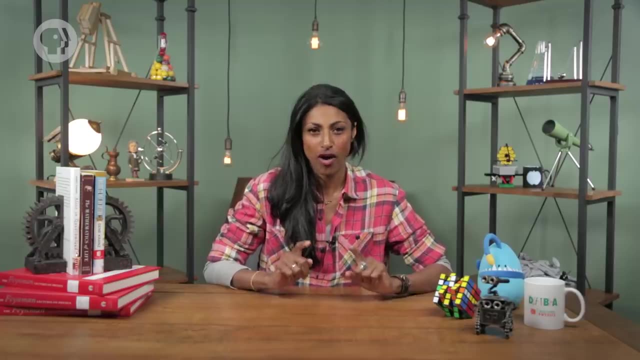 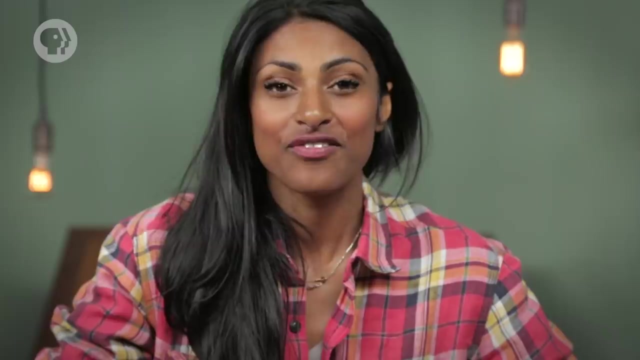 But you don't know the mass that's going through that part of the pipe at any given moment. All you do know are the water's velocity and the area of the cross-section of that certain section of pipe. In order to describe the mass flow rate, you'll have to use what we know about density, area and velocity to work out some algebra magic. 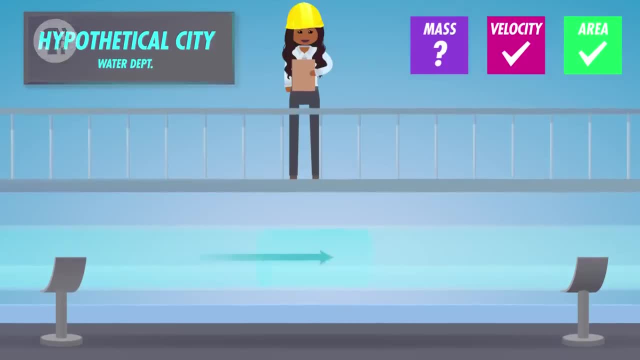 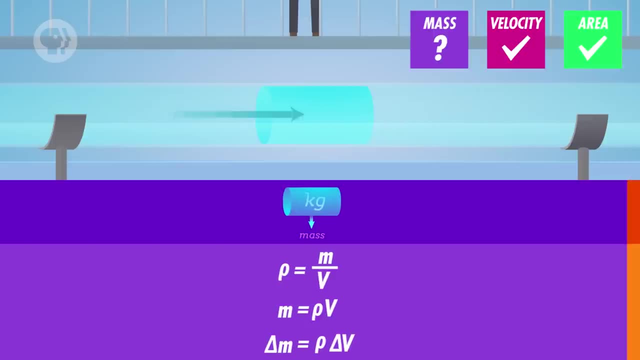 First let's have a look at the cross-section of that point of the pipe. From our last lesson you know that the mass of the fluid moving past this cross-sectional area over time is equal to its density times its volume And the volume of the fluid moving past. this point is simply the area of the pipe at this cross-section. 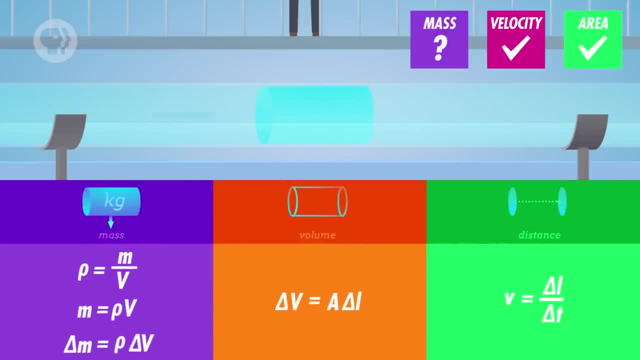 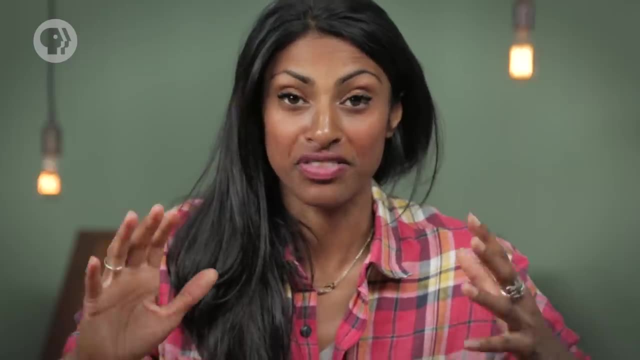 times the distance, the fluid moves. And from our episodes on the physics of motion you'll also know that the distance, the fluid moves divided by the change in time is equal to the fluid's velocity. So by putting that all together you can get a different version of the equation of continuity. 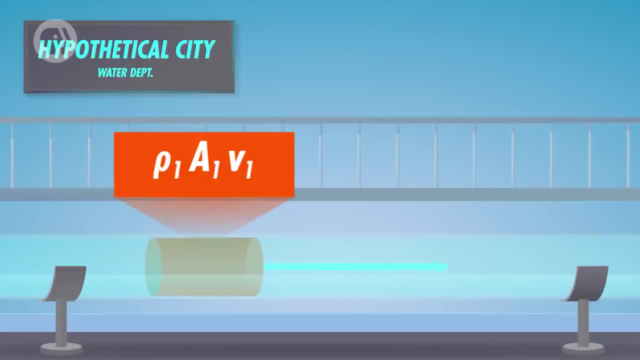 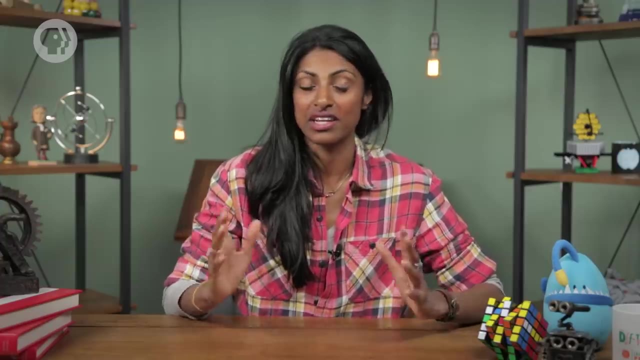 At any given point in the pipe, the density of the fluid flowing through it times the area of the pipe, times the fluid's velocity. will be the same as for any other point in the pipe And since you're dealing with an incompressible fluid, the density is going to be the same for every point in the pipe anyway. 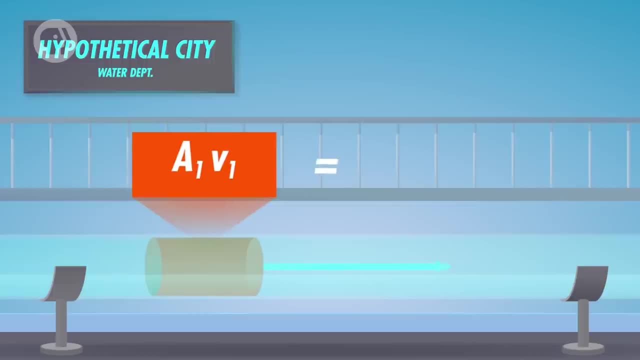 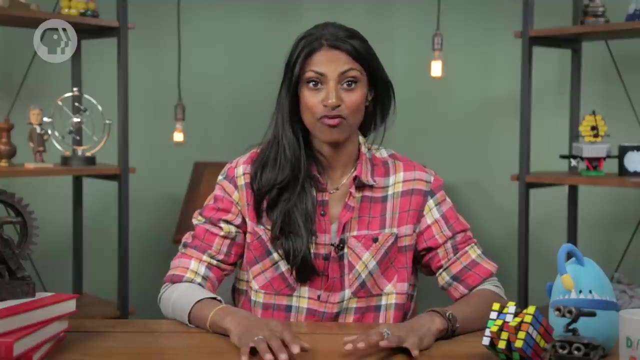 So, really, you've just figured out that at any point in the pipe, the area of the pipe times the fluid's velocity will be the same as for any other point. It's the same thing we said before – the mass flow rate is the same for every point in the pipe. 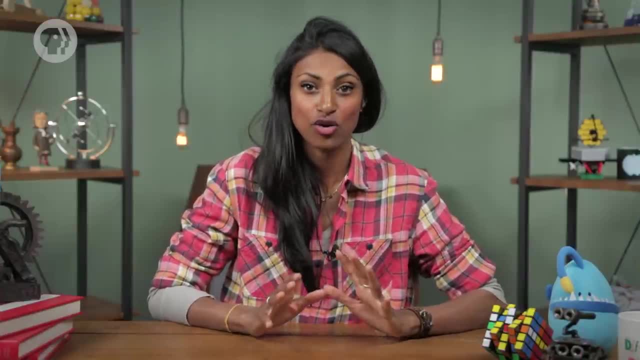 the pipe. That's just because as the water flows through the pipe, it pushes along the water in the rest of the pipe too. So if one part of the pipe has, say, a kilogram of water moving through every second, 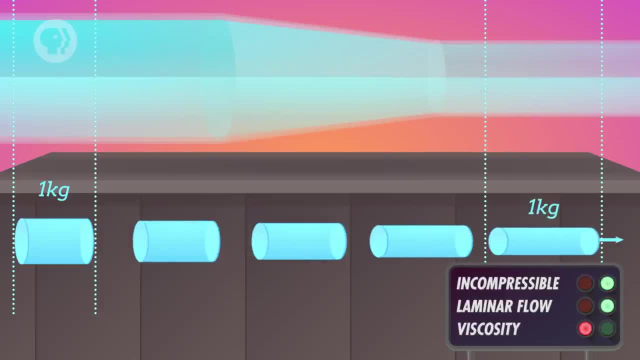 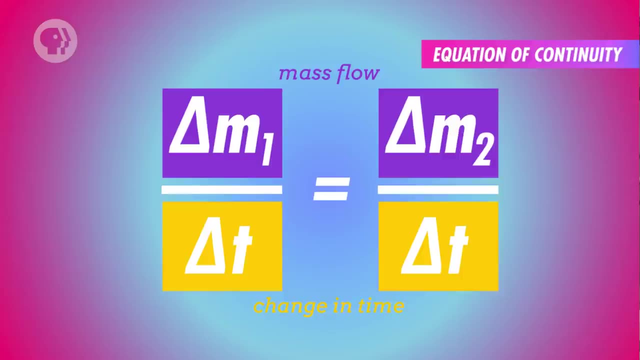 the rest of the pipe also has to have a kilogram of water moving through it every second. To show you another thing: this fact that the mass flow rate at one point of the pipe pipe will be equal to the mass flow rate at any other point is called the equation of continuity. 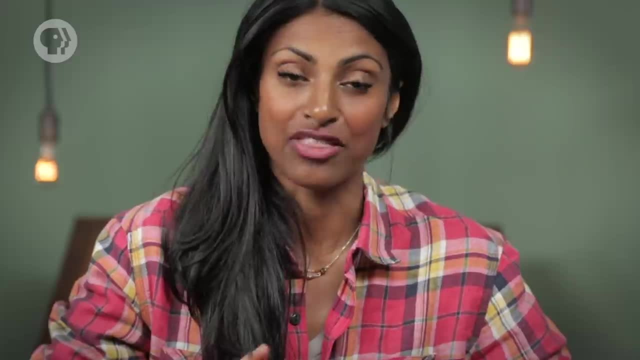 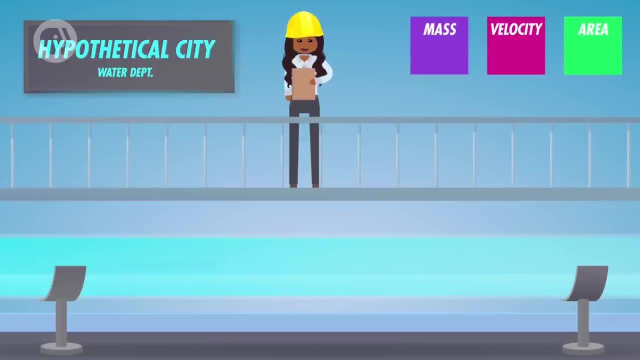 And it can tell you a lot about the relationship between the velocity of a fluid and the cross-sectional area of the pipe that it's flowing through. Let's say you're an engineer for the water department of Hypothetical City and you need to understand the mass flow rate of hypothetical water that's going through a certain point in your underground pipe system. 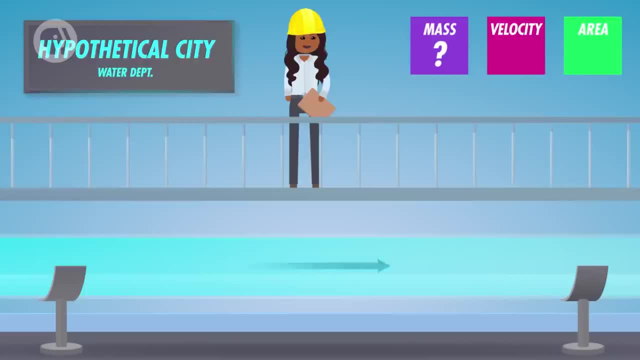 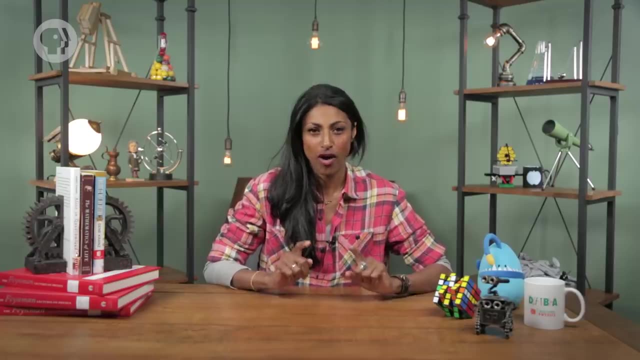 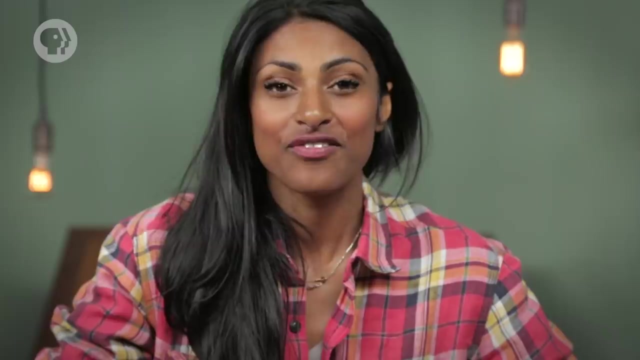 But you don't know the mass that's going through that part of the pipe at any given moment. All you do know are the water's velocity and the area of the cross-section of that certain section of pipe. In order to describe the mass flow rate, you'll have to use what we know about density, area and velocity to work out some algebra magic. 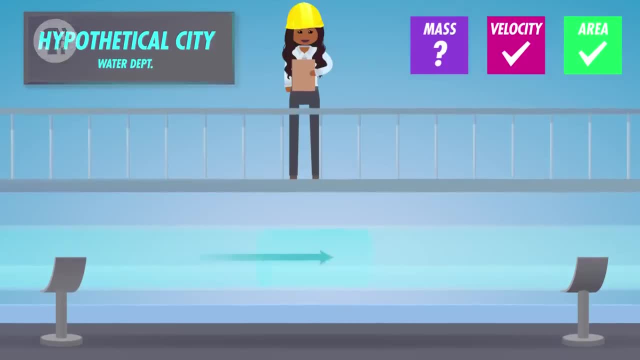 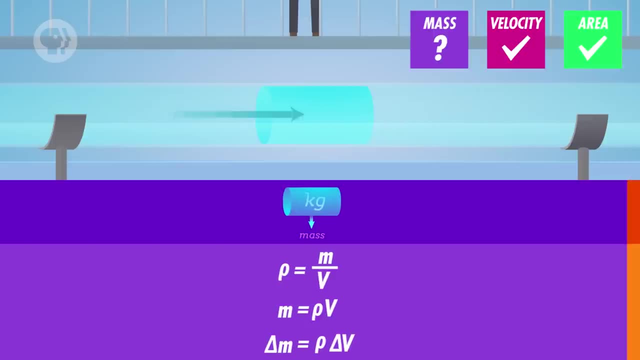 First let's have a look at the cross-section of that point of the pipe. From our last lesson you know that the mass of the fluid moving past this cross-sectional area over time is equal to its density times its volume And the volume of the fluid moving past. this point is simply the area of the pipe at this cross-section. 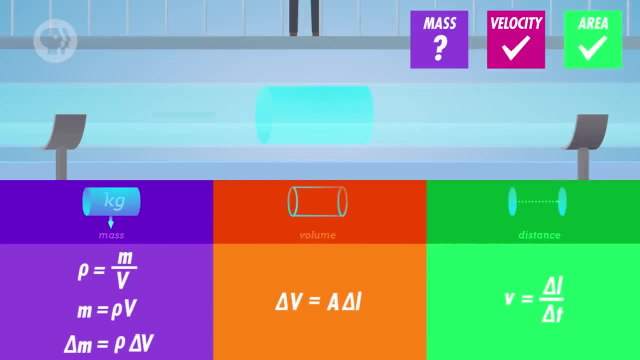 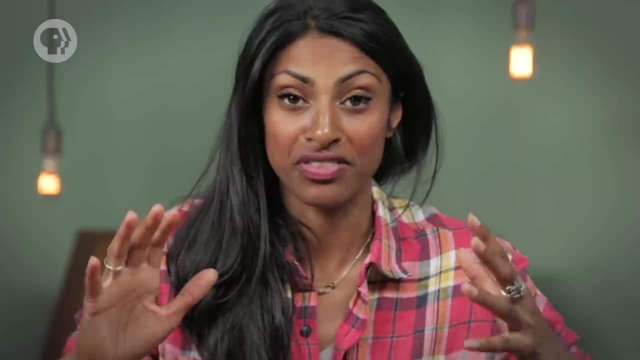 times the distance, the fluid moves. And from our episodes on the physics of motion you'll also know that the distance, the fluid moves divided by the change in time is equal to the fluid's velocity. So by putting that all together you can get a different version of the equation of continuity. 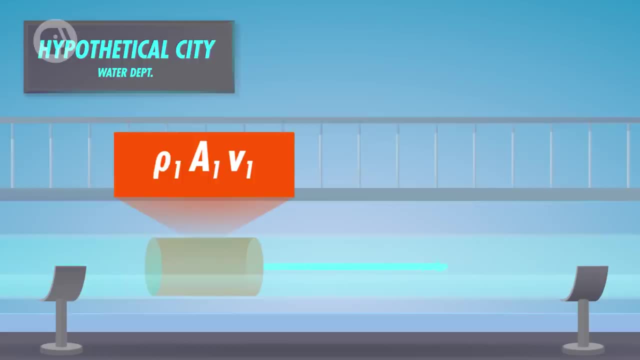 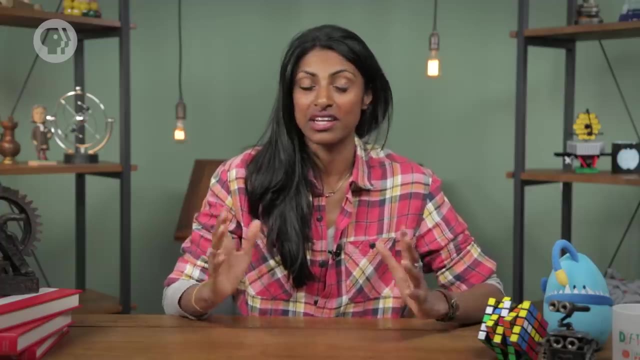 At any given point in the pipe, the density of the fluid flowing through it times the area of the pipe, times the fluid's velocity. will be the same as for any other point in the pipe And since you're dealing with an incompressible fluid, the density is going to be the same for every point in the pipe anyway. 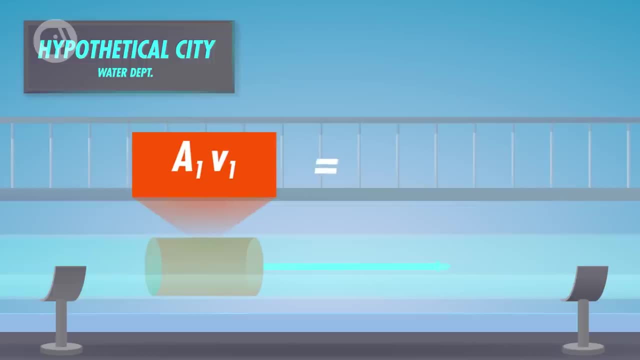 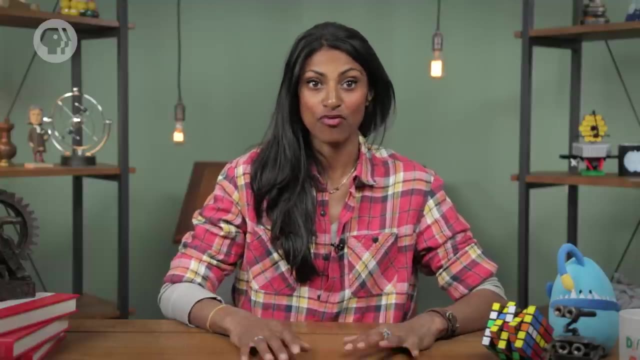 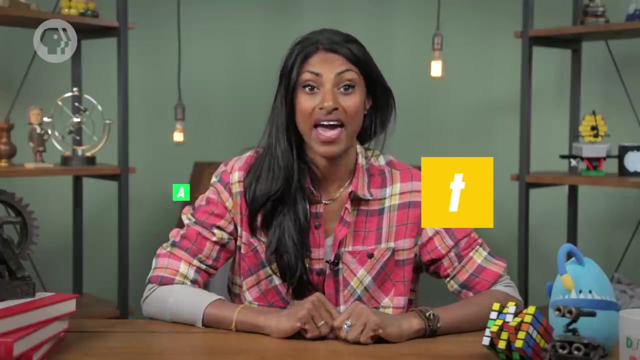 So, really, you've just figured out that at any point in the pipe, the area of the pipe times the fluid's velocity will be the same as for any other point. It's the same thing we said before – the mass flow rate is the same for every point in the pipe. but instead of putting that relationship in terms of mass and time, you're putting it in terms of area and velocity. 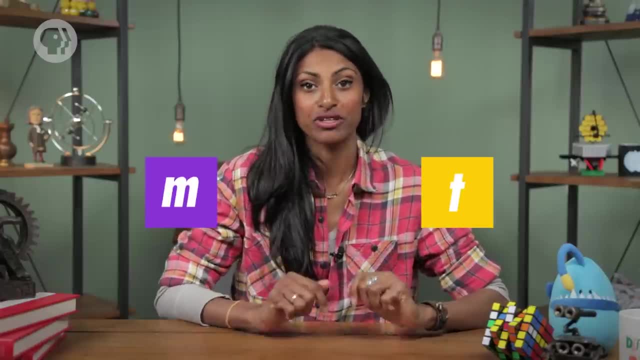 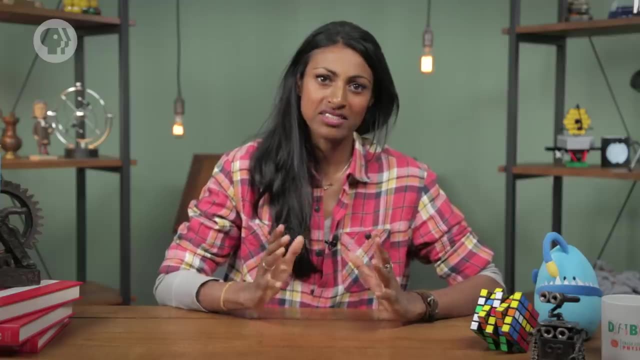 But instead of putting that relationship in terms of mass and time, you're putting it in terms of area and velocity, And in your role as a water department engineer, this is important for you to know, Because it means that where the pipe is narrower, the fluid will have to flow faster in order to compensate. 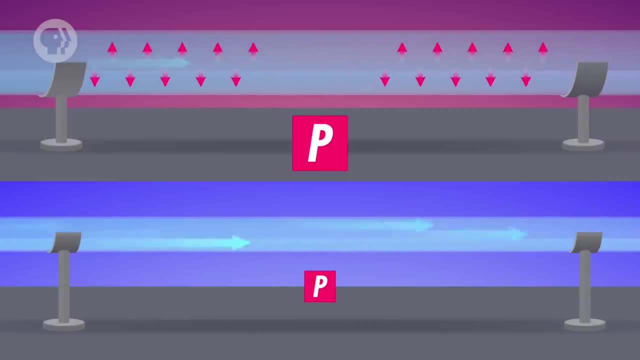 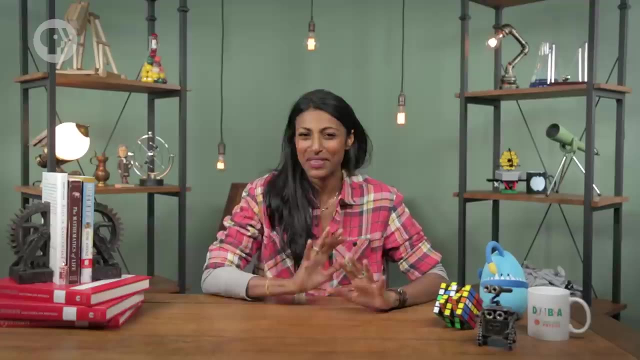 But here's the weird thing: A fluid that's flowing really fast actually has less pressure than when it's flowing more slowly. Sure, it might feel like it's exerting more force than when it flows through a wider opening, But that's not what physicists mean when they talk about the pressure in a pipe. 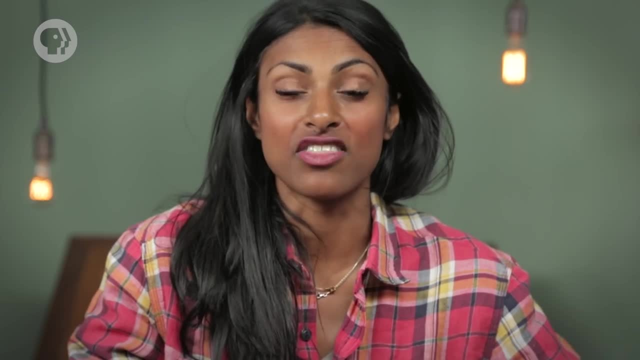 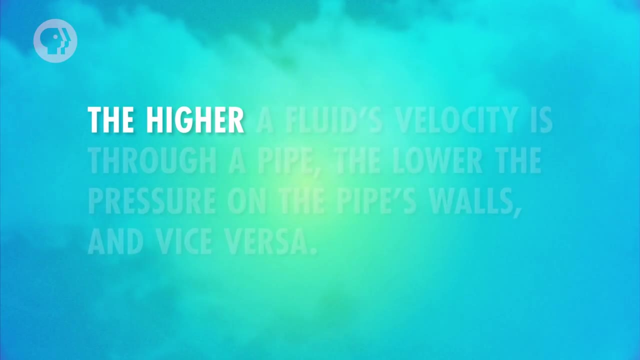 They're really talking about the pressure on the walls of the pipe. This means that the slower the fluid flows, the more pressure it puts on the pipe itself. This is known as Bernoulli's principle. It states that the higher a fluid's velocity is through a pipe, the lower the pressure on the pipe's walls, and vice versa. 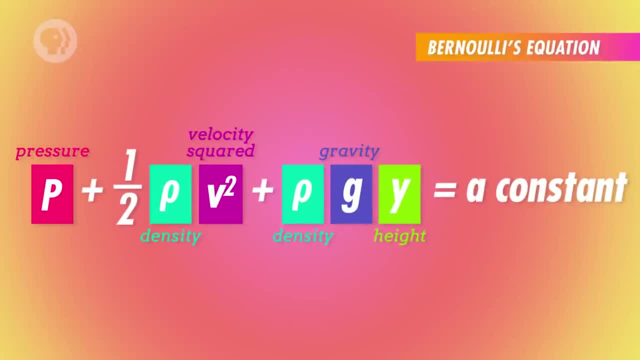 Bernoulli also came up with what we now know as Bernoulli's equation. It might look kind of intimidating at first, but when you break it down it's actually just a way of combining a bunch of things that you've already learned. 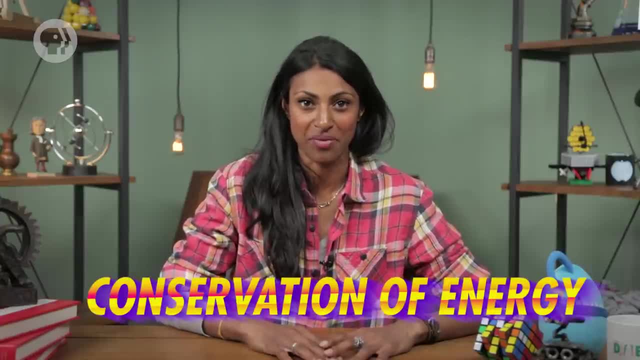 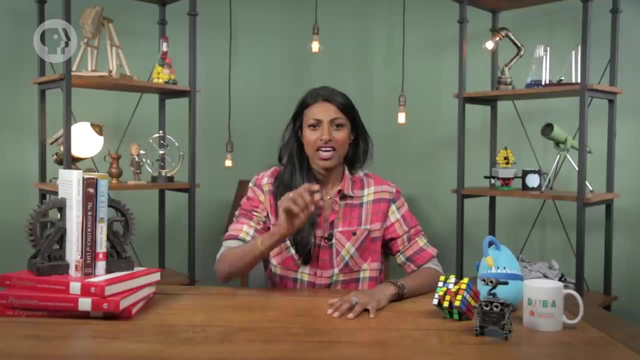 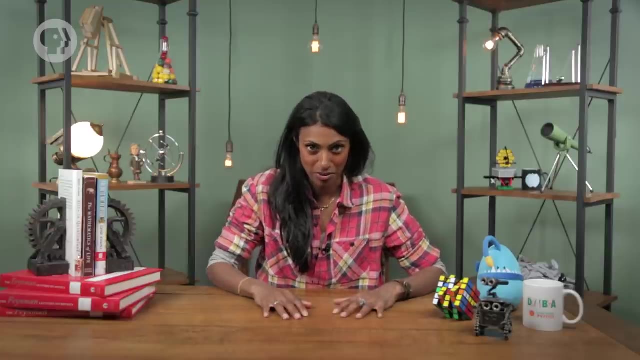 Bernoulli based his equation on the concept of the conservation of energy. As a fluid flows through a pipe, it won't gain or lose energy. This means that no matter where the fluid is in the pipe, if you take all the forms of energy that the fluid has at that point and add them up, they'll equal the same number as any other point in the pipe. 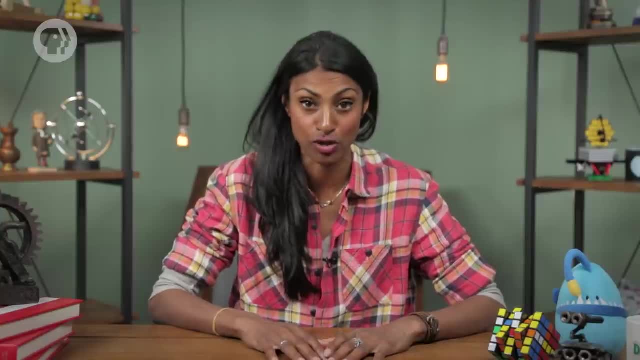 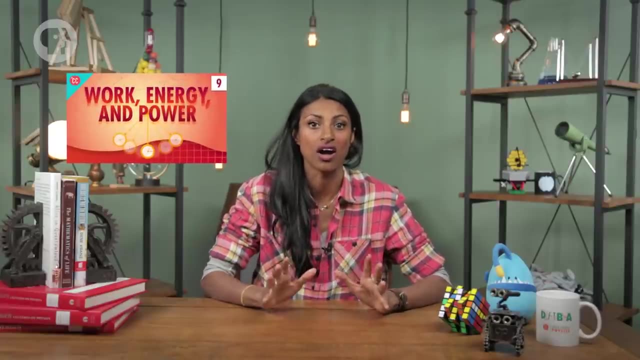 Have a look at how the three forms of energy in a fluid are represented in Bernoulli's equation. First there's pressure, times, volume. In our episode on work and energy, we defined energy as the ability to do work, And when a fluid applies pressure and moves the volume of fluid that's downstream, it's doing work. 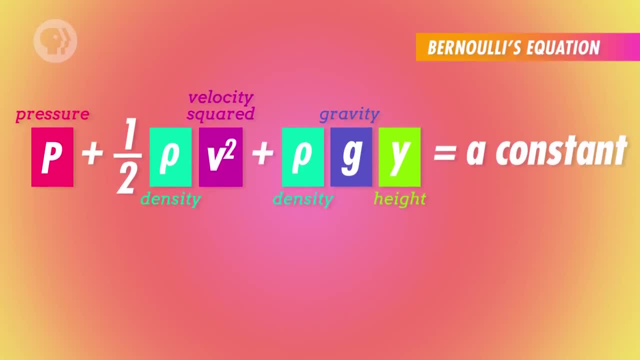 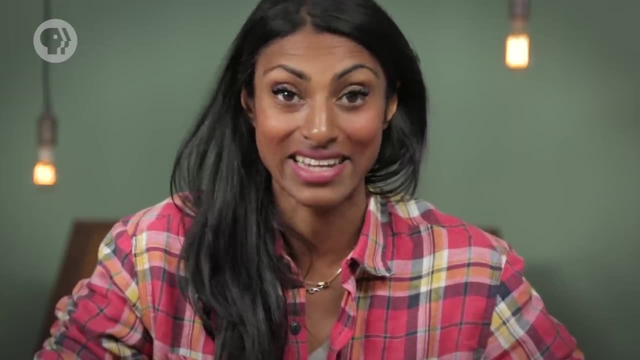 So pressure times volume must be a form of energy. The first term in Bernoulli's equation takes that energy and divides it by volume, which just leaves pressure. Next, a flowing fluid also has kinetic energy. When we first talked about kinetic energy we said that the flow of energy is the flow of energy. 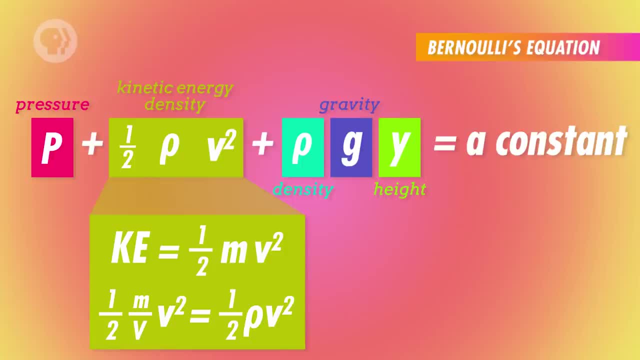 We said that it's equal to half of an object's mass times its velocity squared. Again, Bernoulli divided this form of energy by volume to get half the fluid's density times its velocity squared. That's called the kinetic energy density and it's the second term of Bernoulli's equation. 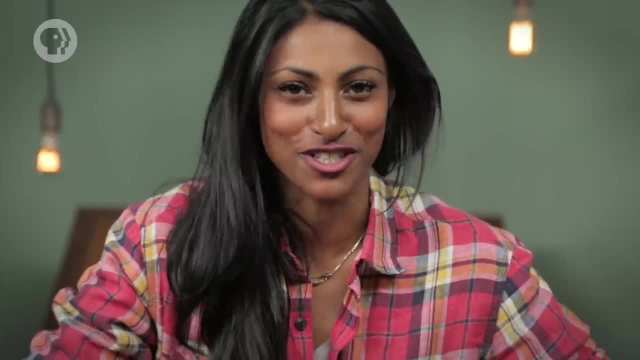 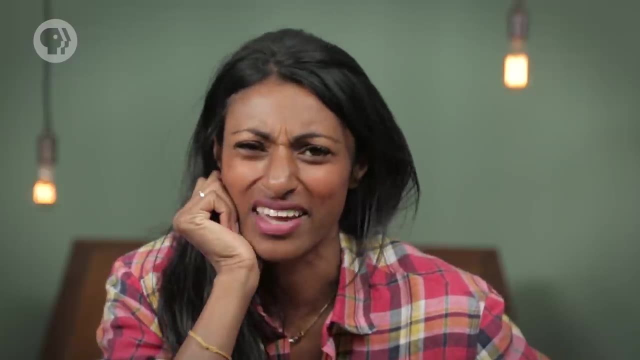 And in your role as a water department engineer, this is important for you to know, Because it means that where the pipe is narrower, the fluid will have to flow faster in order to compensate. But here's the weird thing: A fluid that's flowing really fast actually has less pressure than when it's flowing more slowly. Sure, it might feel like it's exerting more force than when it flows through a wider opening, but that's not what physicists mean when they talk about the pressure in a pipe. They're really talking about the pressure on the walls of the pipe. 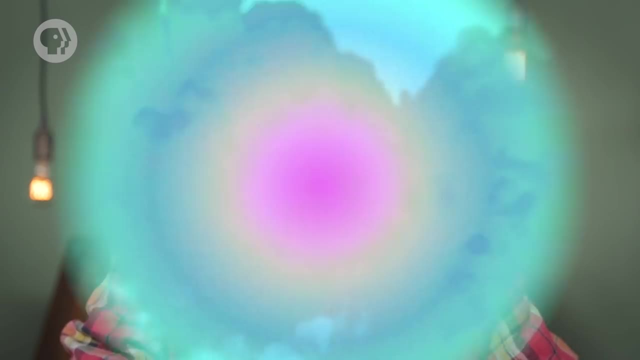 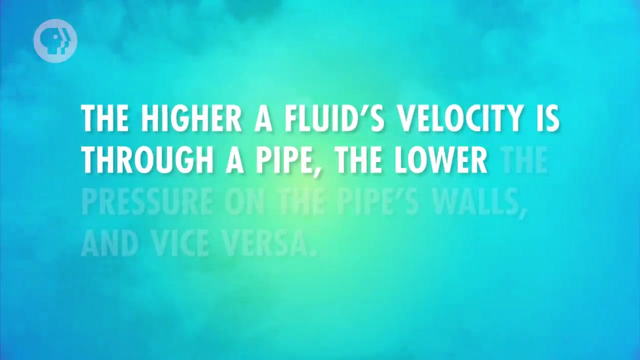 This means that the slower the fluid flows, the more pressure it puts on the pipe itself. This is known as Bernoulli's Principle. It states that the higher a fluid's velocity is through a pipe, the lower the pressure on the pipe's walls, and vice versa. 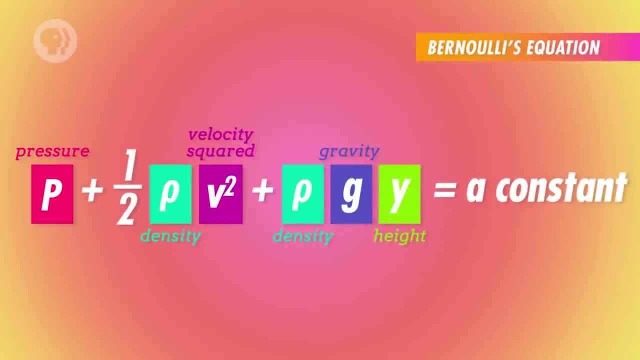 Bernoulli also came up with what we now know as Bernoulli's Equation. It might look kind of intimidating at first, but when you break it down it's actually just a way of combining a bunch of things that you've already learned. 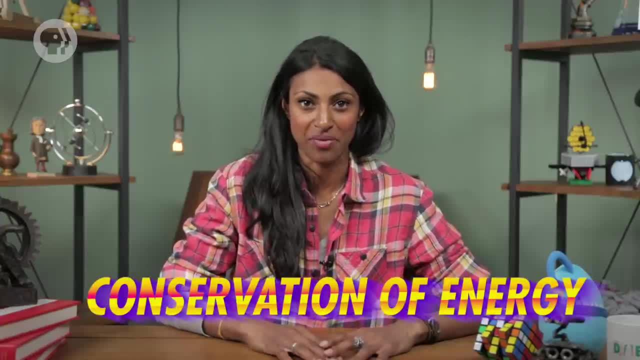 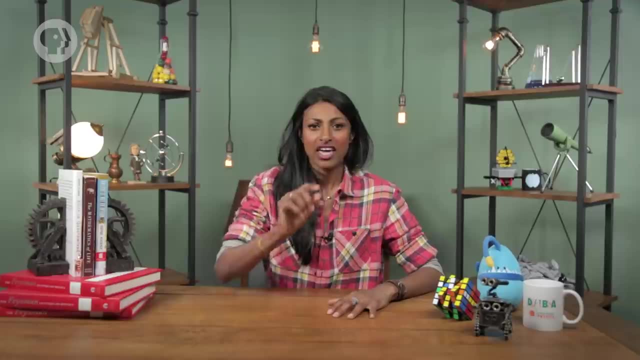 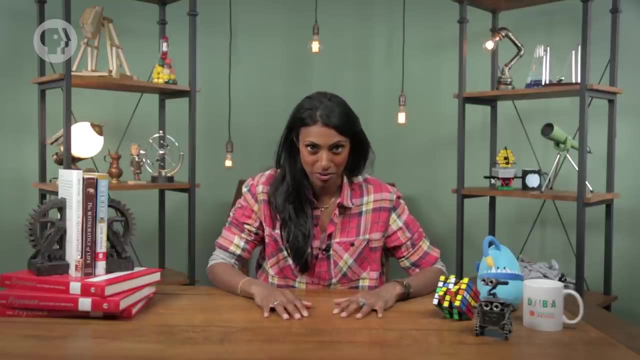 Bernoulli based his equation on the concept of the conservation of energy. As a fluid flows through a pipe, it won't gain or lose energy. This means that no matter where the fluid is in the pipe, if you take all the forms of energy that the fluid has at that point and add them up, they'll equal the same number as any other point in the pipe. To better understand this, we can use the equation to calculate the flow of energy. To do this, have a look at how the three forms of energy in a fluid are represented in Bernoulli's equation. First, there's pressure, times, volume. 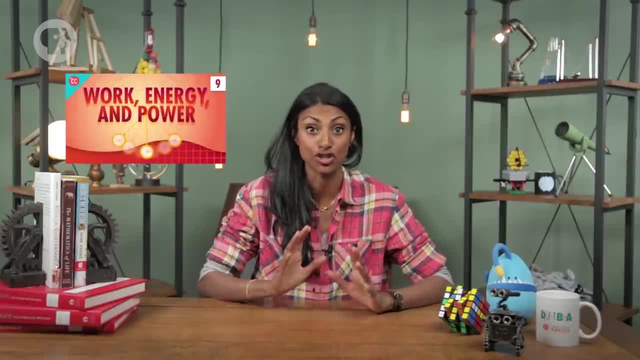 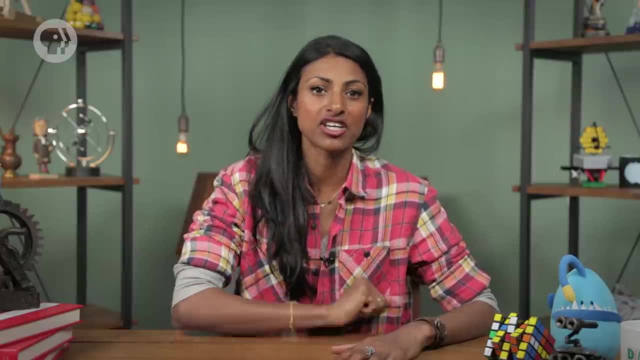 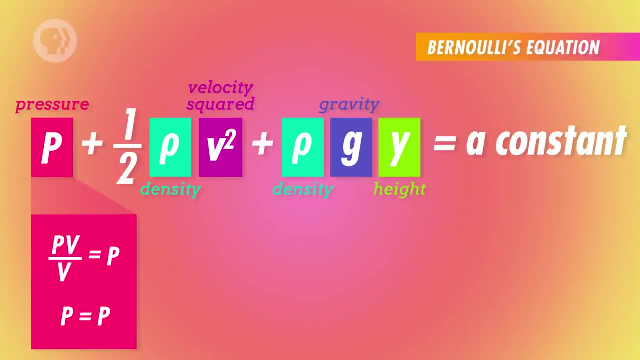 In our episode on work and energy, we defined energy as the ability to do work, And when a fluid applies pressure and moves the volume of fluid that's downstream, it's doing work. So pressure times volume- must be a form of energy. The first term in Bernoulli's equation takes that energy and divides it by volume, which just leaves pressure. 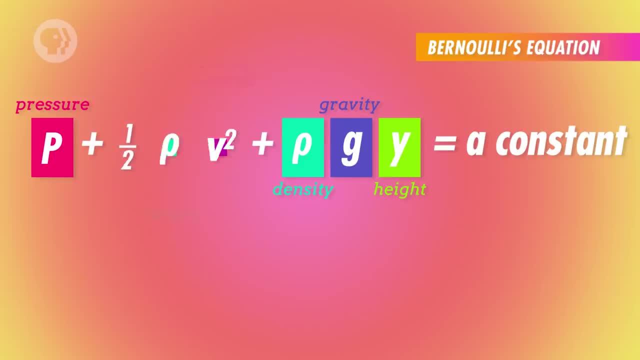 Next, a flowing fluid also has kinetic energy. When we first talked about kinetic energy, we saw that the flow of energy has a kinetic energy. He said that it's equal to half of an object's mass times its velocity squared. Again, Bernoulli divided this form of energy by volume to get half the fluid's density times its velocity squared. 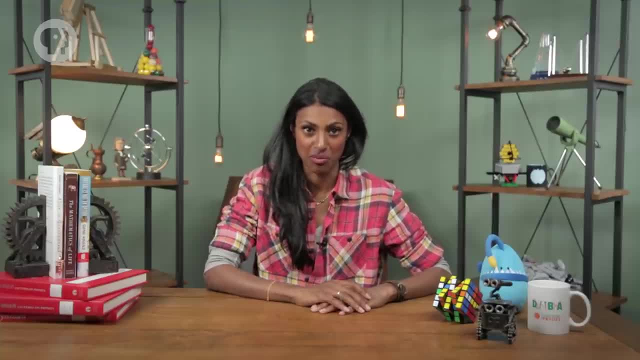 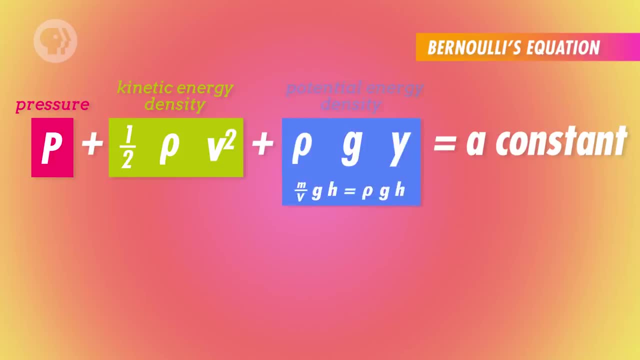 That's called the kinetic energy density and it's the second term of Bernoulli's equation. Finally, a flowing fluid also has the potential energy that comes from gravity, And we've said before that the potential energy from gravity is equal to an object's mass times small g times its height. 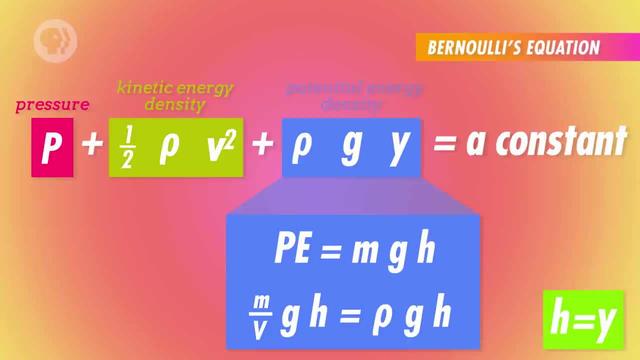 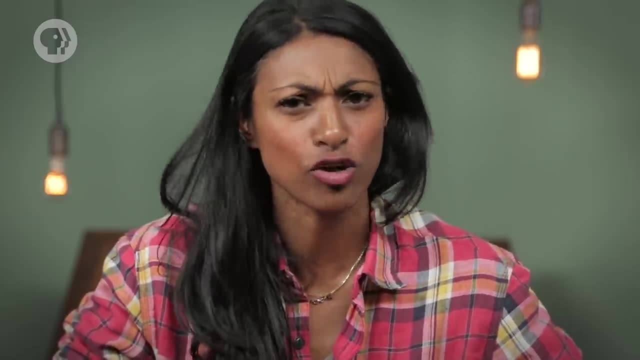 When Bernoulli divided that by volume, he got density times, small g times, height, the potential energy density and the third term of his equation. Why divide all these terms by volume? Well, when it comes to fluids, it's just easier to talk about things in terms of density than it is to talk about mass. 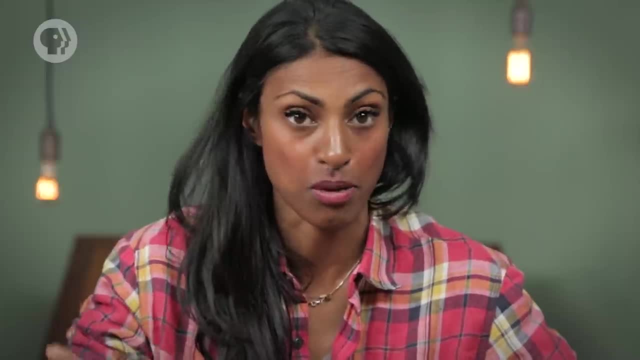 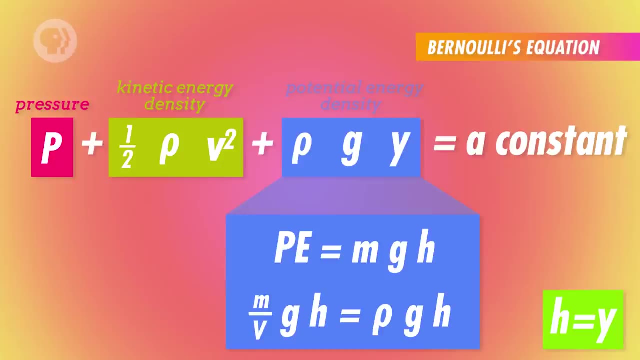 Finally, a flowing fluid also has the potential energy that comes from gravity, And we've said before that the potential energy from gravity is equal to an object's mass times small g times its height. When Bernoulli divided that by volume, he got density times volume. 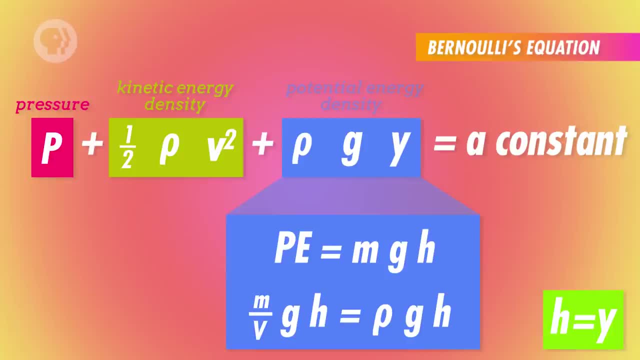 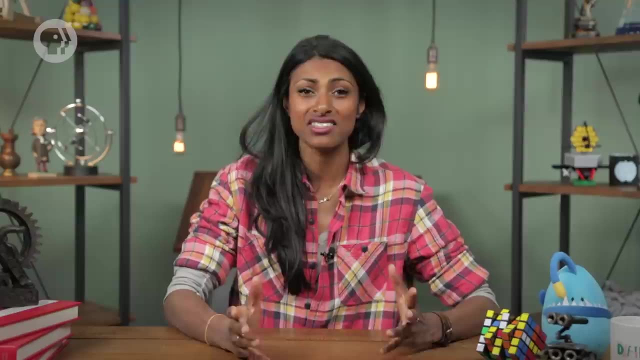 He got density times, small g times height, the potential energy density and the third term of his equation. Why divide all these terms by volume? Well, when it comes to fluids, it's just easier to talk about things in terms of density than it is to talk about mass. 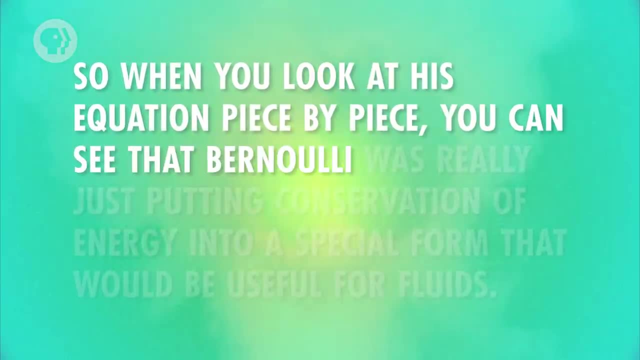 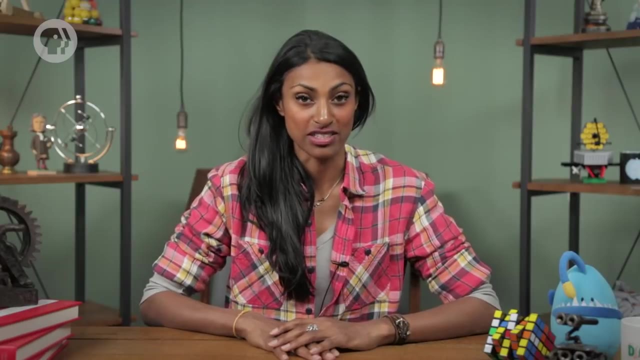 So when you look at his equation piece by piece, you can see that Bernoulli was really just putting conservation of energy into a special form that would be useful for fluids. Now let's look at a special case of Bernoulli's equation, known as Torricelli's theorem. 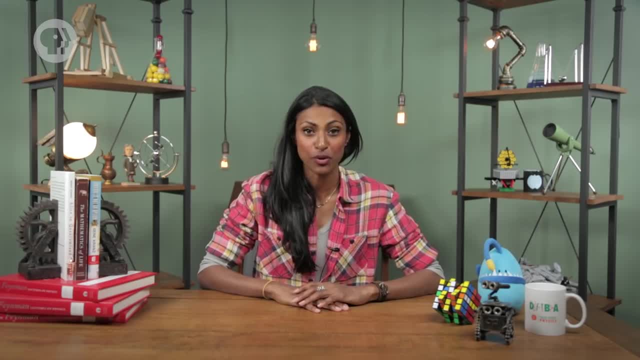 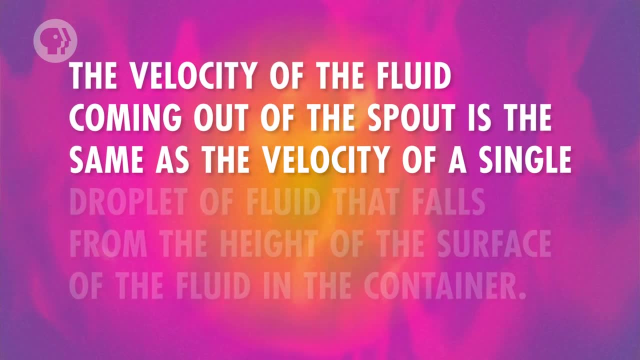 Torricelli's theorem uses conservation of energy to find the volume of fluid. It uses this energy to find the velocity of fluid flowing from a small spout in a container, And it says that the velocity of the fluid coming out of the spout is the same as the velocity of a single droplet of fluid that falls from the height of the surface of the fluid in the container. 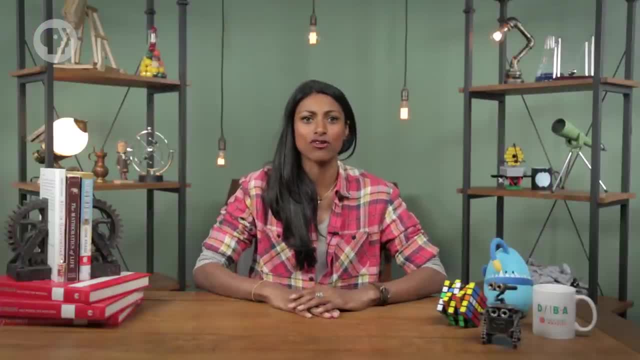 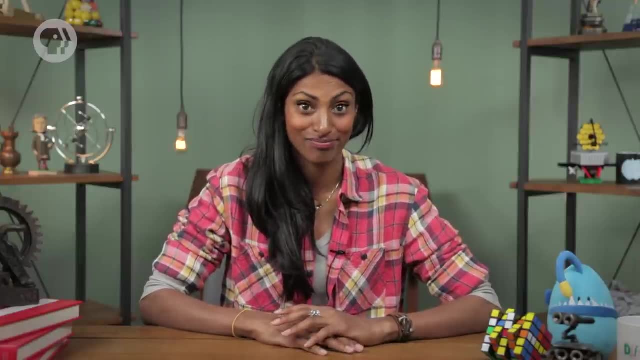 In other words, the pressure that's pushing the fluid out of the spout gives it the same velocity that it would get from the force of gravity. To see this theorem in action, let's say you're not a water department engineer, you're just… you. 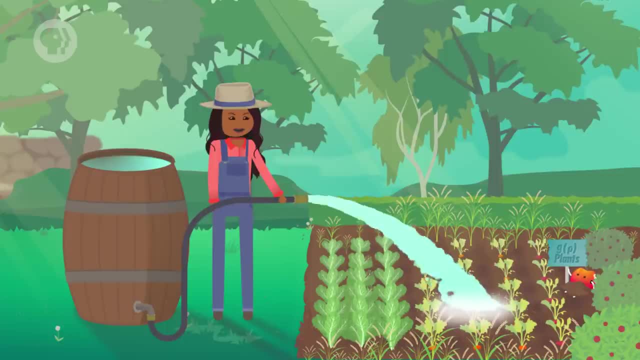 And you're watering your garden with the water you've saved up in your rain barrel. Your barrel doesn't have a top And you're watering your carrots and lettuce instead. And you're watering your garden with the water you've saved up in your rain barrel. 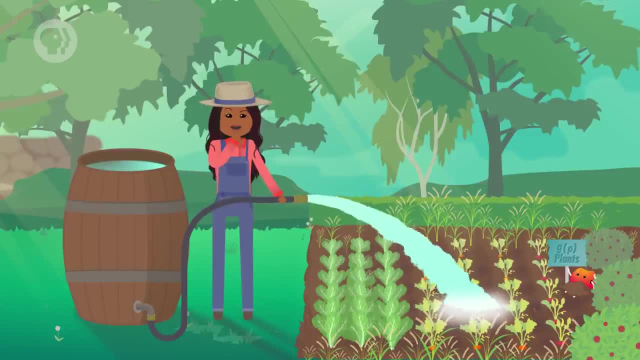 And you're watering your carrots and lettuce instead, And you're watering your carrots and lettuce instead, And you're watering your carrots and lettuce instead. You so many times have to start from a hole or a spout in the side. Now you want to know what the velocity is of the water coming out of the spout. 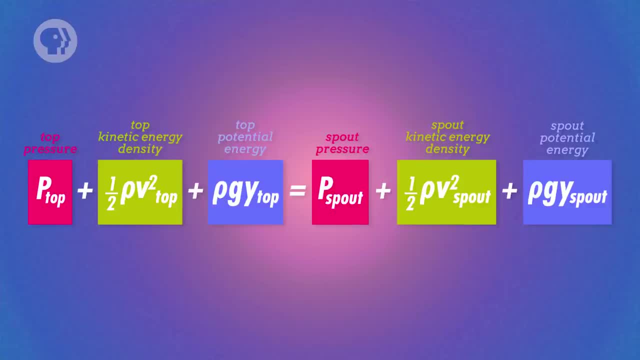 From Bernoulli's equation we know that the sum of the pressure, kinetic energy density and the potential energy density of the water at the top of the barrel will equal the sum of those three qualities of the water coming out of the spout. 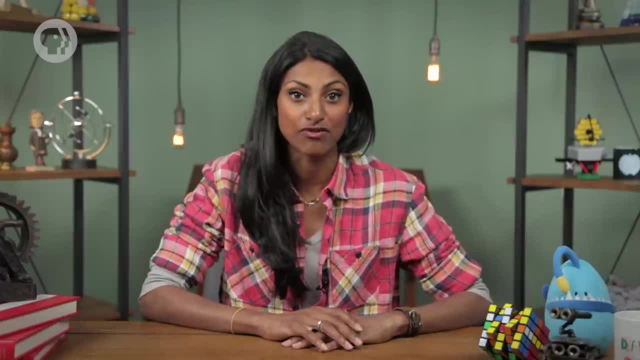 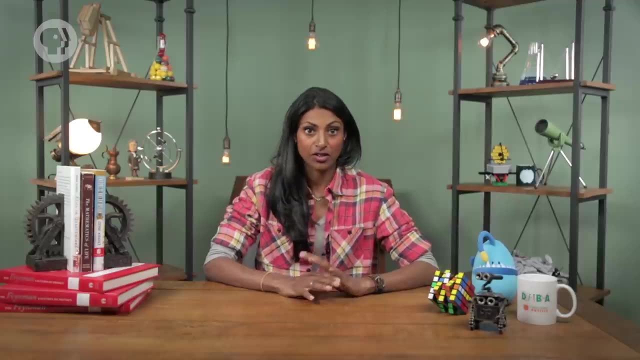 But we can simplify that relationship a bit to find the velocity of the fluid coming out First. the upper surface of the water in the barrel and the water that's coming out of the spout are both exposed to the atmosphere, So the pressure at those points will be the same. 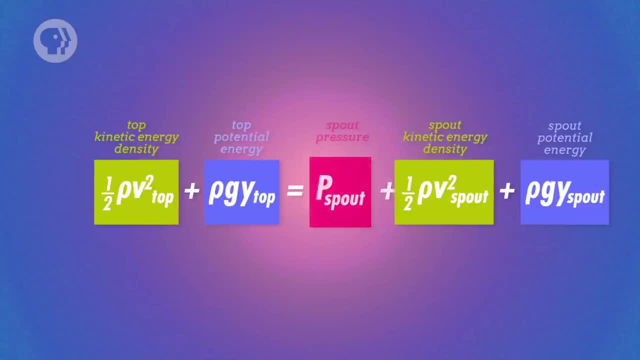 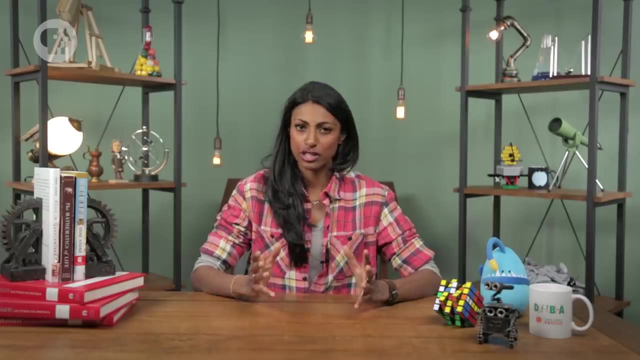 will be the same. it's just atmospheric pressure, So we can cross off the pressure from each side of the equation. Now there might be water coming out of the spout, but the top of the barrel has a much bigger area, So the water at the top of the barrel isn't going to be moving much. 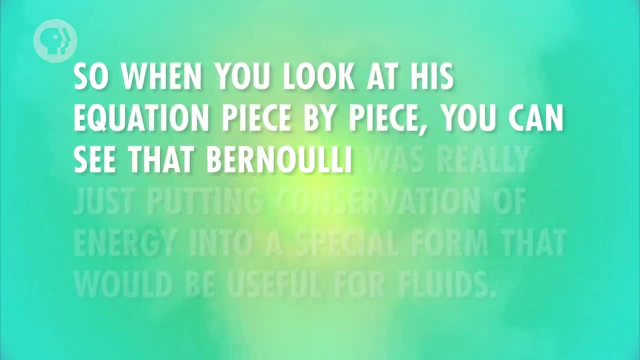 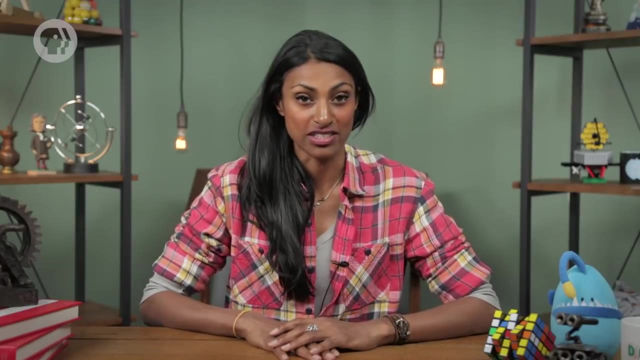 So when you look at his equation piece by piece, you can see that Bernoulli was really just putting conservation of energy into a special form that would be useful for fluids. Now let's look at a special case of Bernoulli's equation, known as Torricelli's theorem. 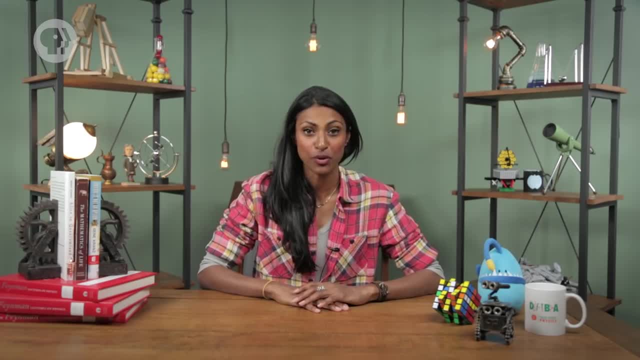 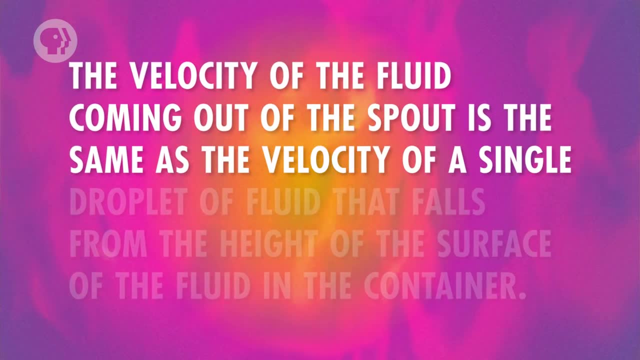 Torricelli- Torricelli. Torricelli- Torricelli's theorem uses conservation of energy to find the velocity of fluid flowing from a small spout in a container, And it says that the velocity of the fluid coming out of the spout is the same as the velocity of a single droplet of fluid that falls from the height of the surface of the fluid in the container. 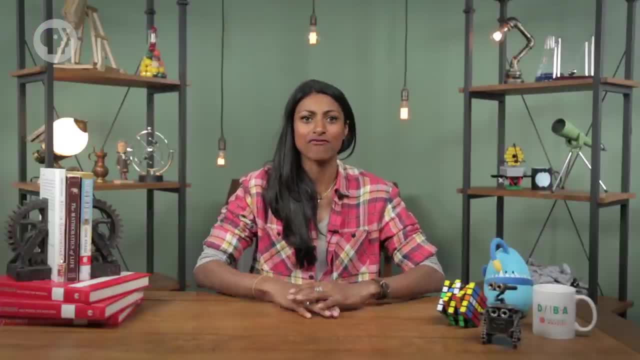 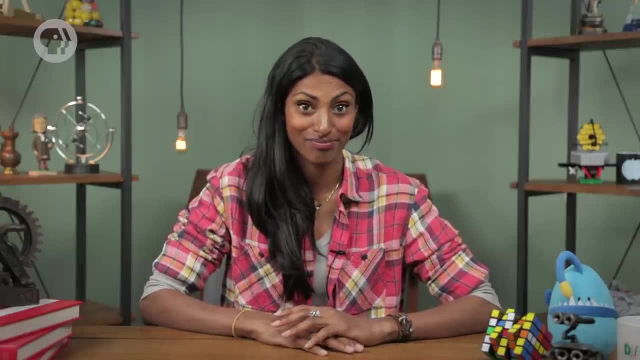 In other words, the pressure that's pushing the fluid out of the spout gives it the same velocity that it would get from the force of gravity. To see this theorem in action, let's say you're not a water department engineer, you're just… you. 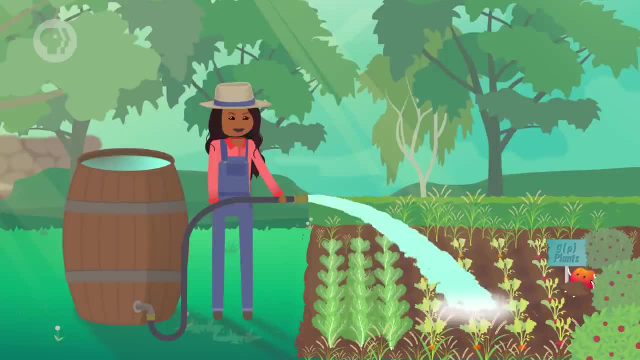 And you're watering your garden with the water you've saved up in your rain barrel. Your barrel doesn't have a top And you're watering your carrots and lettuce and stuff from a hole or a spout in the side. Now you want to know what the velocity is of the water coming out of the spout. 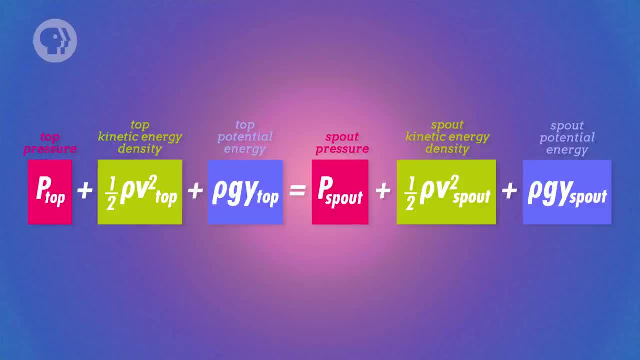 From Bernoulli's equation we know that the sum of the pressure, kinetic energy density and the potential energy density of the water at the top of the barrel will equal the sum of those three qualities of the water coming out of the spout. 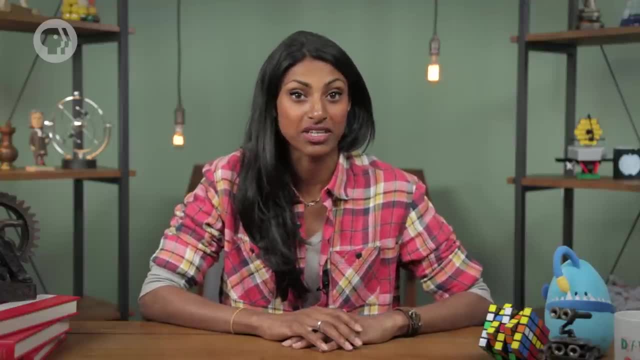 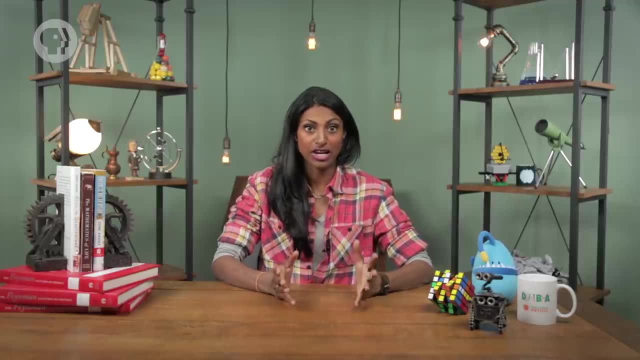 But we can simplify that relationship a bit to find the velocity of the fluid coming out First. the upper surface of the water in the barrel and the water that's coming out of the spout are both exposed to the atmosphere. The pressure at those points will be the same. it's just atmospheric pressure. 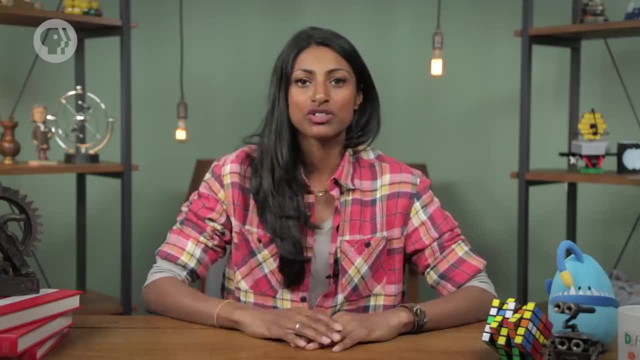 So we can cross off the pressure from each side of the equation. Now there might be water coming out of the spout, but the top of the barrel has a much bigger area, So the water at the top of the barrel isn't going to be moving much. 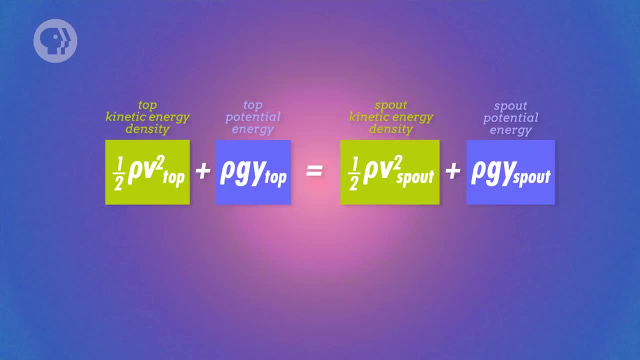 In fact, we can say that its velocity is basically zero, Which means that the kinetic energy density for the water at the top of the barrel is zero. Finally, we can cross out the density in each term of the equation, since it's not changing. 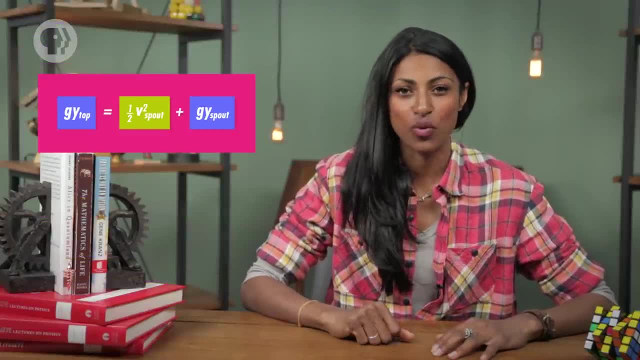 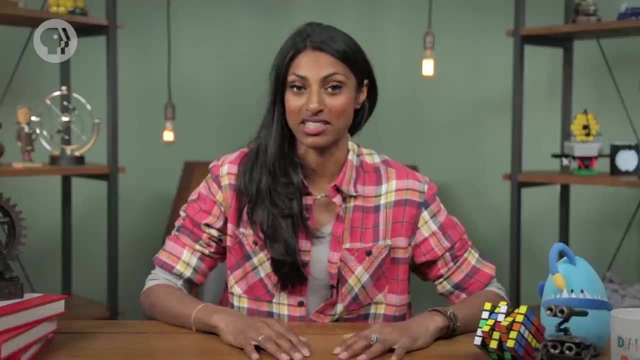 We're left with a much simpler equation with only three terms, An equation that should look very familiar if you watched our episodes on the physics of motion. It's a kinematic equation. You already know the two main kinematic equations: the definition of acceleration and the displacement curve.